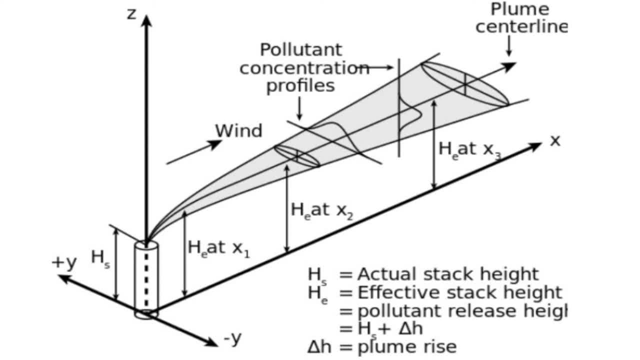 Welcome. In this video we are talking about Gaussian plume model, which is about the dispersion model for pollutants as a point source, like the one coming out of a stack or a chimney- What this graph is all about. This graph represents Gaussian model of plume dispersion. To understand the graph in a better fashion, we will go to the following video and after that we will come back to this graph. 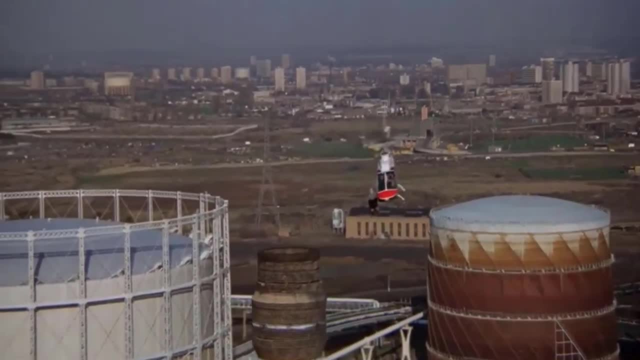 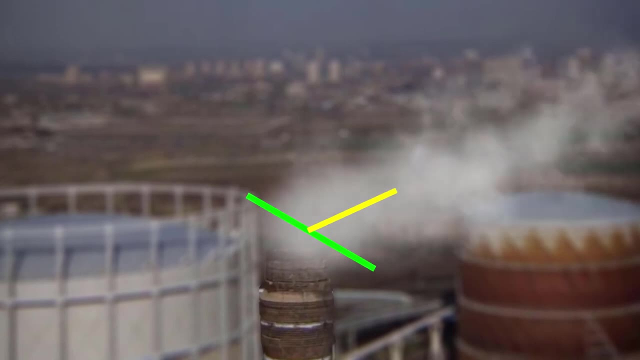 Okay, hope you enjoy the James Bond movie clip. Center of attraction of the clip is a stack or a chimney And on seeing the video you must have an idea about the height of the stack. Also, please note now the plume is coming out of the stack, Wind is also flowing. Wind direction is towards the tank, as you see on the right hand side. 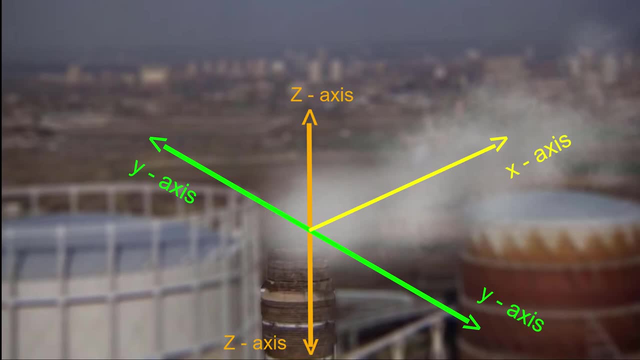 So plume is also flowing in the same direction. So that is our x-axis. Otherwise, x-axis is the plume direction as well as the wind direction. And now the wind is uniform, say maybe with a velocity capital U. we may denote it. 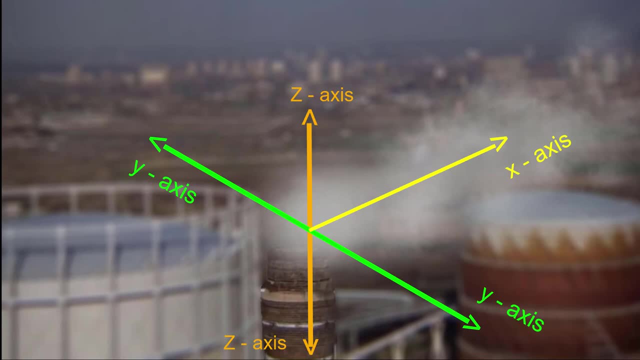 Now please also note the transverse direction denoted by the green axis, or called y-axis, which is transverse to the plume. Also note the vertical axis passing through the stack, which is called the z-axis. So these are the x-axis. 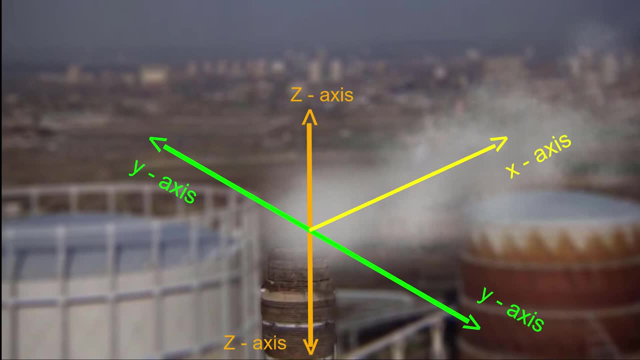 So these are the x, y and z-axis with respect to a plume dispersion. You can also see we have an oval, blue oval there, which represent the cross section of the plume. This may be circular, may be irregular, whatever, depending on the type of plume. So now we are bothered about the concentration across this particular cross section. 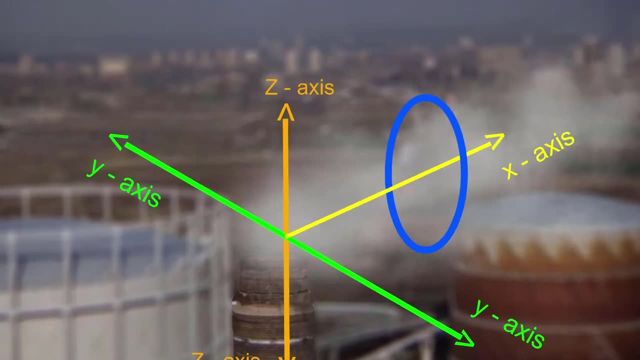 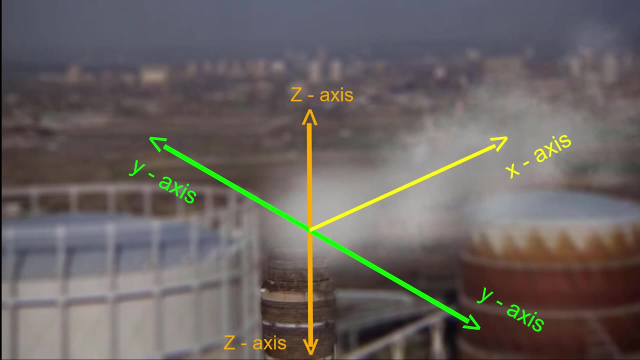 That is, a concentration of pollutants across this particular cross section. And also, please note The x-axis which is starting from the plume discharge location, or that is the point source, and it is directed towards the windward direction or downwind direction. 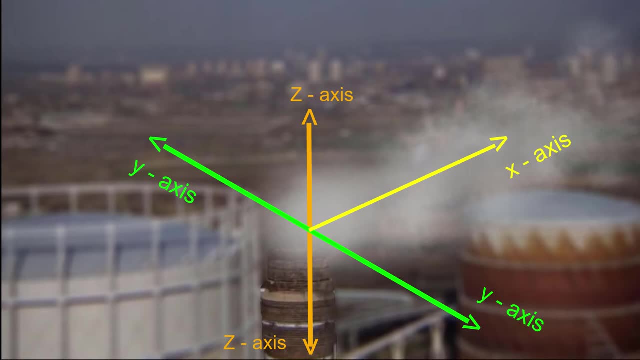 And also note that the y-axis, or the transverse axis- it is growing towards the left as well as right. The meaning of this is the particle from the center of plume may move either to the left or right as it spreads, or as it moves downwards. 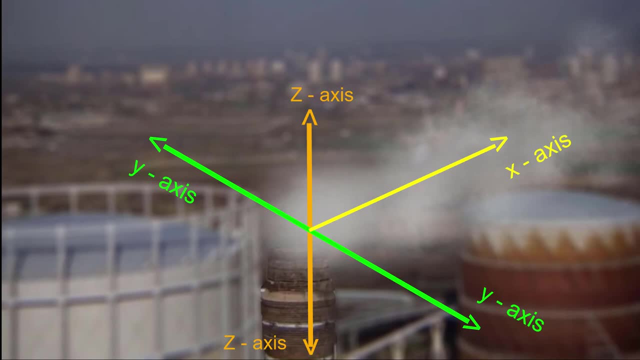 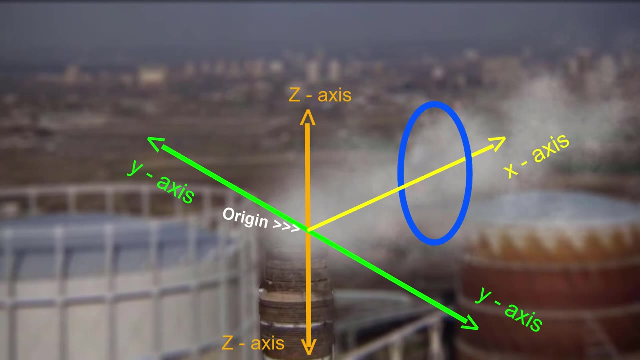 So from the west. that is when the particle moves around the wind. Similarly the z-axis also. it is also growing up as well as down, from the origin, whatever we have considered The origin as a discharge point. So from the origin, uh x, uh, sorry, z-axis is so moving up and down. 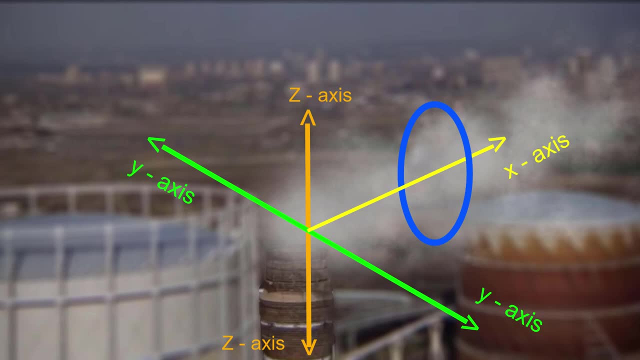 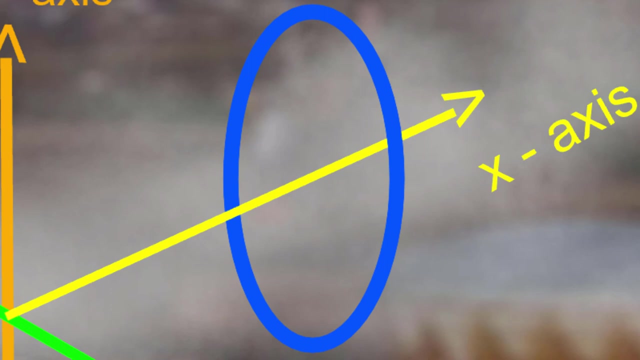 This means that the particles, as it travels, may move up or down. So to represent represent these particles, dispersion, we have plus y minus y-axis, as well as plus z minus z-axis. Now We may have to see how the concentration of pollutant is distributed across a given or a particular cross section. 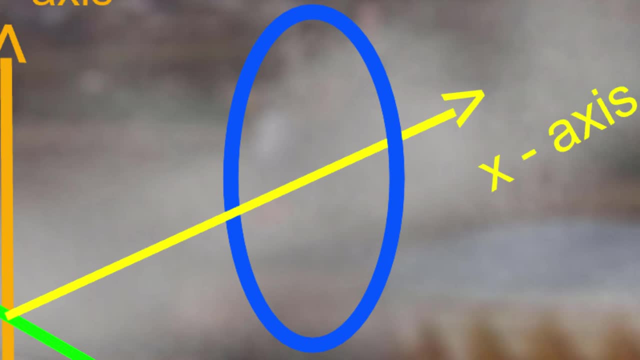 Here we make an assumption. or in Gaussian plume model, the assumption is: the concentration from the center of plume at a given cross section varies according to normal distribution. So here the possibility of variation at a given cross section. Given cross section is at a distance x1 from the origin or the discharge point. 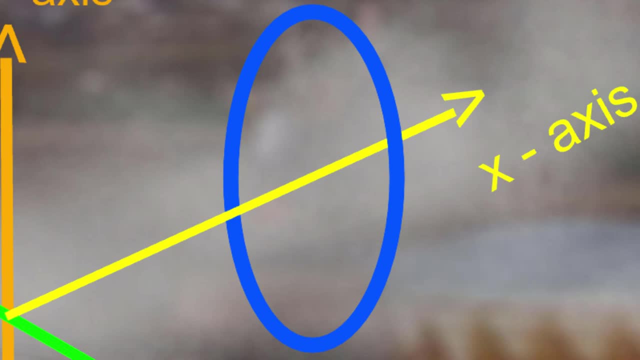 So at this location x1, the variation along the cross section can be either one the variation along y-axis and second the variation along z-axis. So there is a double distribution. We have a double distribution across the cross section of the plume. 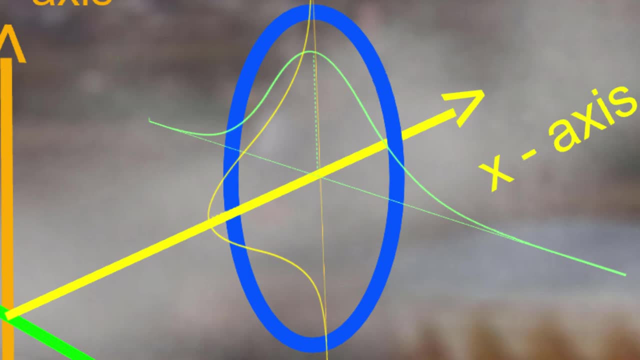 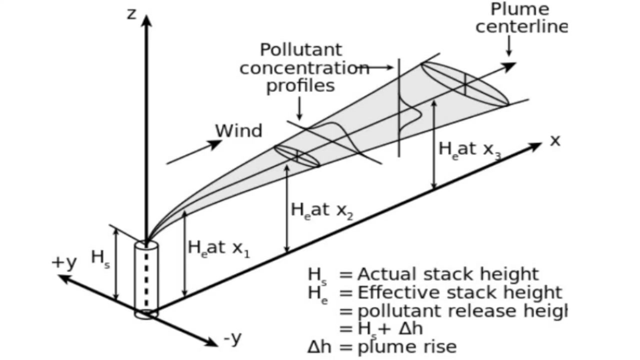 One is in y-axis, other is in z-axis. So we can see two normally distributed graph here. One is directed based on the y-axis, other is directed based on the z-axis. So now you may note various parameters in this particular graph. 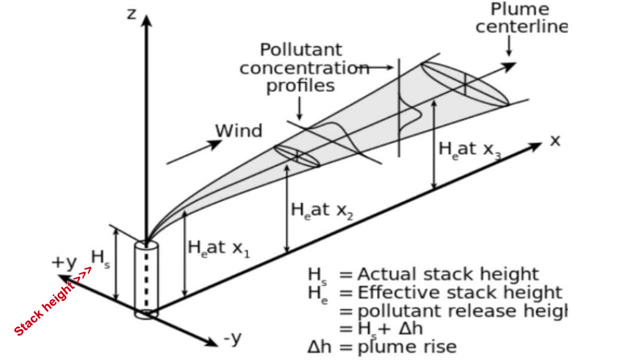 Height of stack is hs and at various locations, at x1, x2, x3, etc. along the x-axis The height is hs, Termed as effective stack height, That is hs plus delta h, which is plume rise, may be momentum rise or whatever rise.